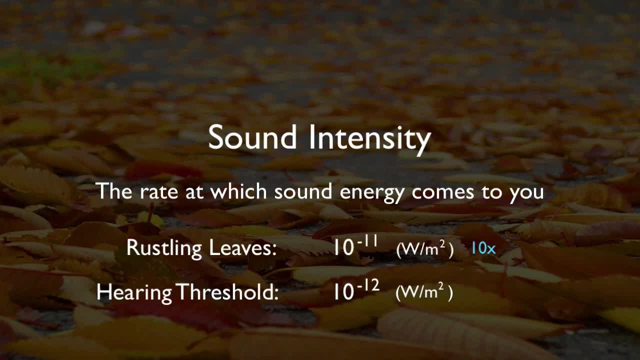 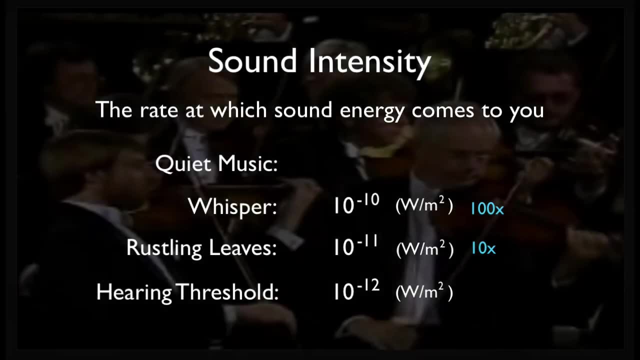 sidewalk has an intensity of about 10 times as great. A whisper is a hundred times as intense, But quiet radio music playing in the background, that's about 10,000 times as intense. So let's think about that. Quiet music, from an energy standpoint, is about 10,000 times as intense as the smallest sounds we can hear. 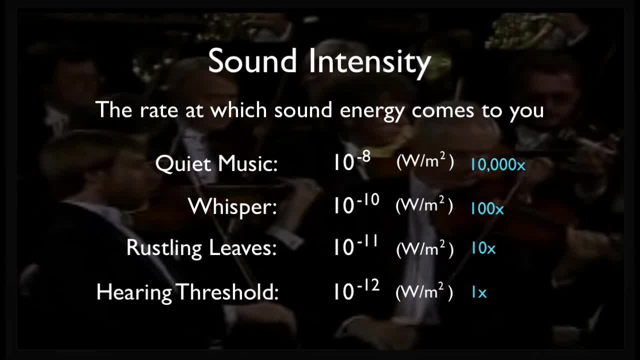 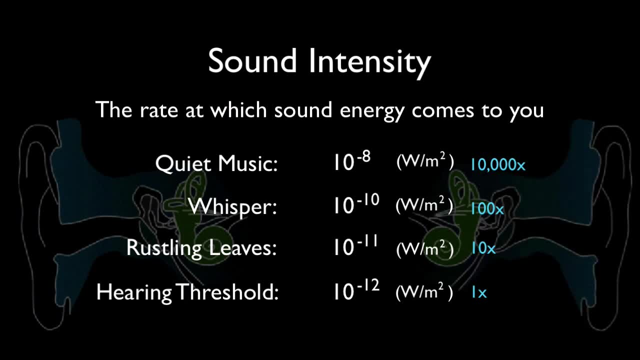 So why doesn't it feel like 10,000 times as intense? Answer: the human ear is sensitive to a very, very broad range of sound intensities. Only 10,000 times as intense is nothing. My voice right now is about a million times as intense as the sound intensity. 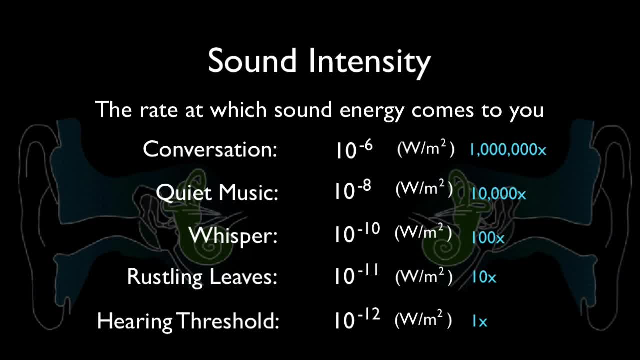 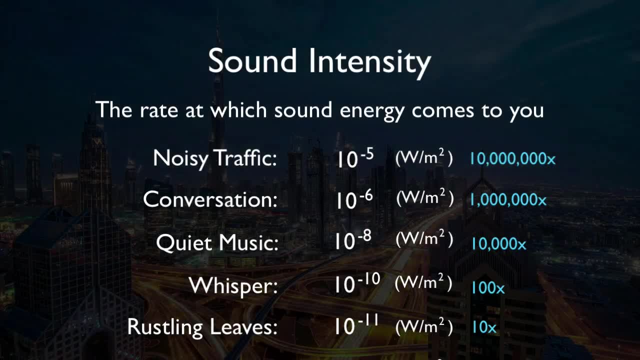 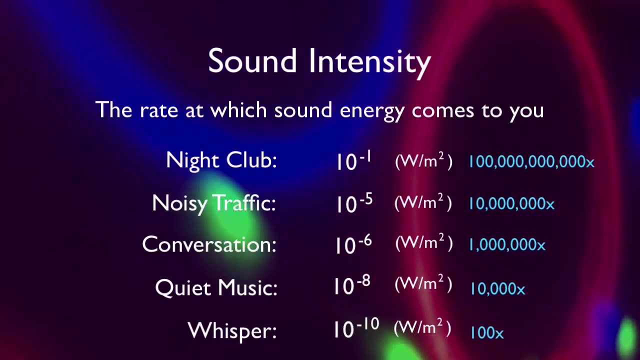 This music should be about 10 million times as intense. as the smallest sound. we can detect Noisy city traffic. That's about 10 million times as powerful. What about loud music at a nightclub? Well, that's about 100 billion times as intense. 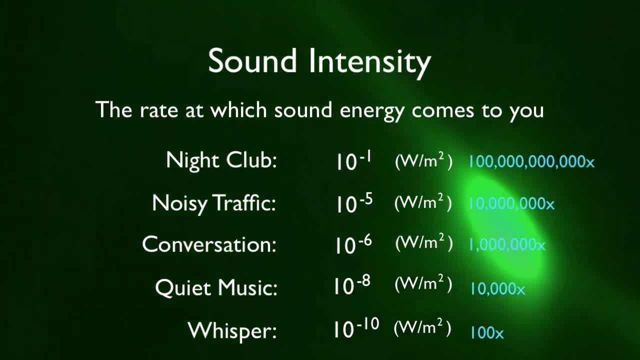 We're talking a huge range. The human ear is designed to deal with a very huge range of sound intensities. That's only 100 to the minus. It's a huge amount louder than I'm thinking of when people talk loud music, And so it can become something that happens to me all the time. 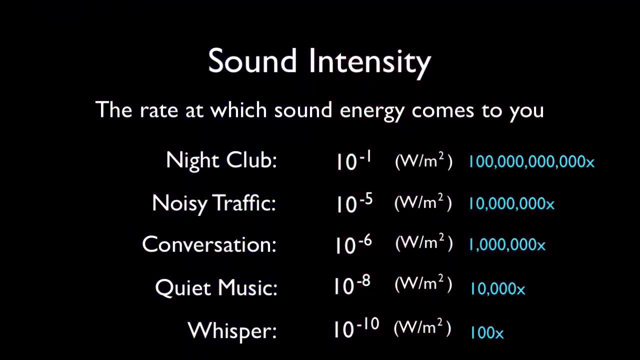 We're talking about two or three hundred times or so as intense Noisy city traffic. That's about 10 million times as powerful big numbers. And big numbers, as you know, can be unwieldy. So that's why sound level is typically. 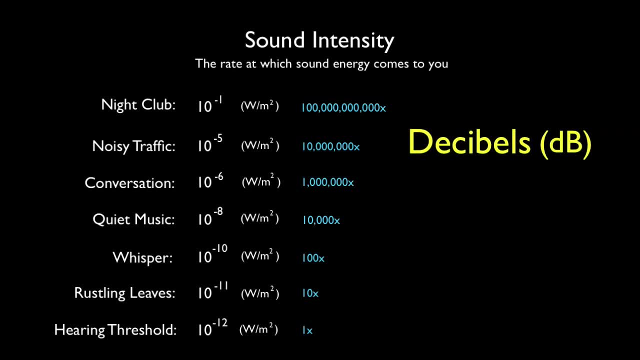 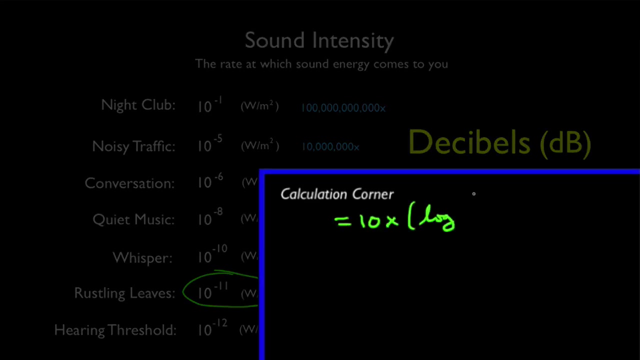 given in units called decibels. A decibel is defined as 10 times the log of the ratio of a given sound to the smallest sound. Let's do an example: The rustle of leaves has a sound intensity of 10 to the minus 11th watts per square meter. Take this and divide it by the smallest sound. we. 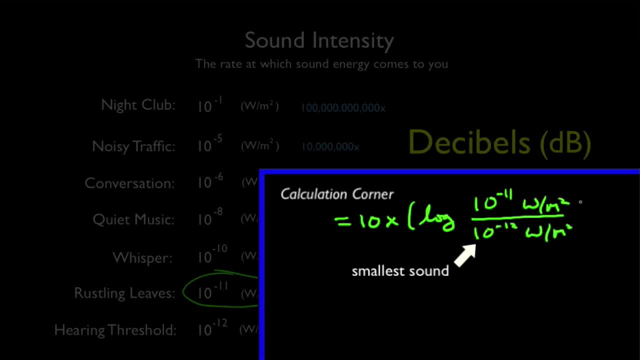 can hear, which is 10 to the minus 12th watts per square meter, and you get 10 to the first. Recall that when you divide numbers with exponents, you just subtract the exponents to get the answer. So what's the log of 10 to the 1?? Logs are actually quite simple With a log. 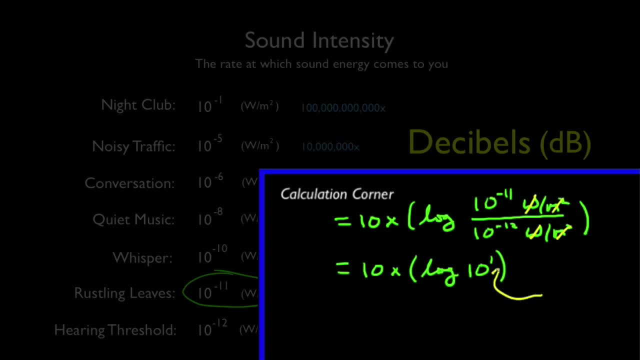 you're merely asking: to what power is 10 raised? Do you see here that 10 to the first is 10 raised to the 1?? So to what power is 10 raised? The answer is 1.. The log of 10 to the 1 is 1.. So take 10 times. 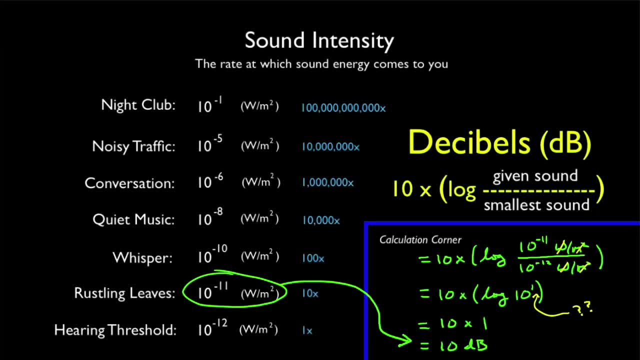 that and you have 10 decibels. The intensity of rustling leaves is about 10 decibels. Let's do an example. Another example: How about a whisper 10 to the minus 10, divided by 10 to the minus 12? 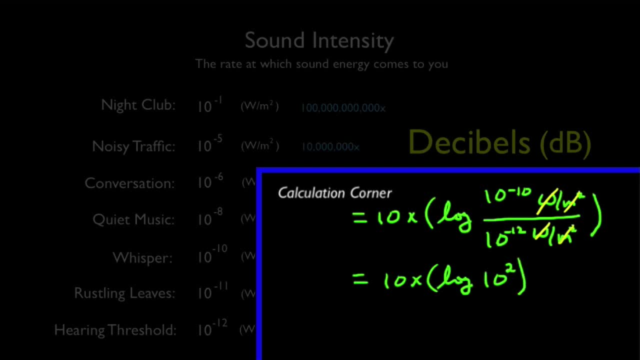 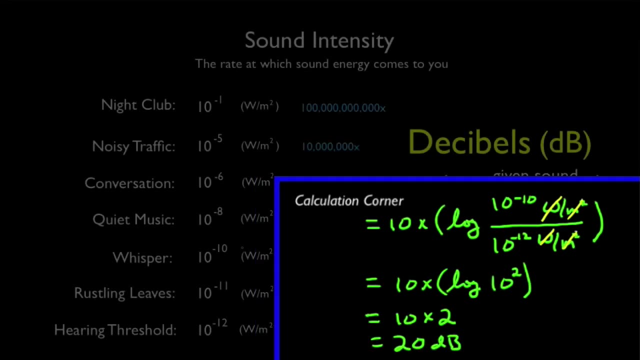 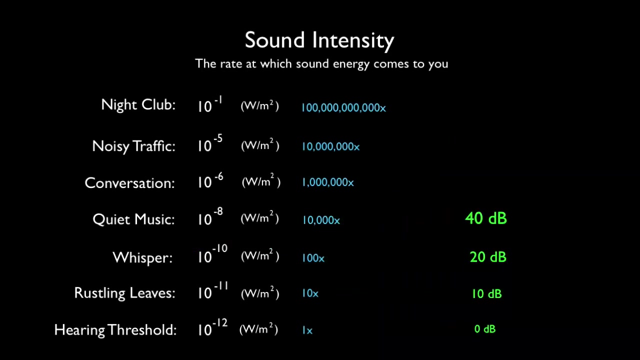 is 10 to the 2.. What's the log of 10 to the 2?? The answer is 2.. 10 times that and you have 20 decibels. By the same math, quiet music is about 40 dB. My voice is about 60 dB. A busy street. 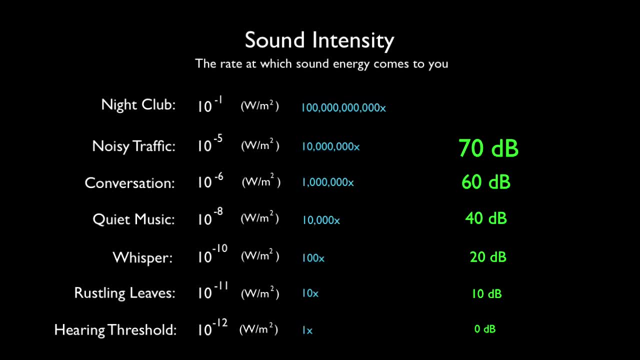 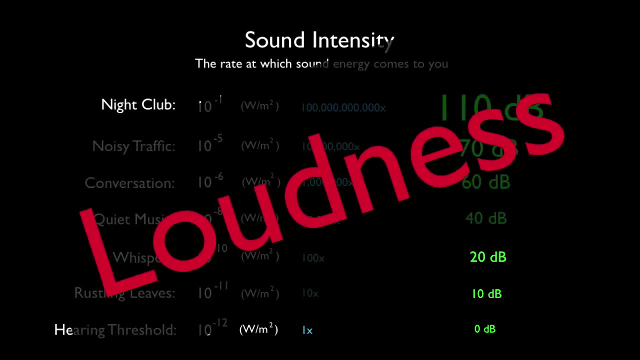 which is 10 times as intense, comes in at 70 dB. A blaring disco comes in at an astounding 110 dB or decibels, And this brings up the idea of loudness, While sound intensity is a physical characteristic. 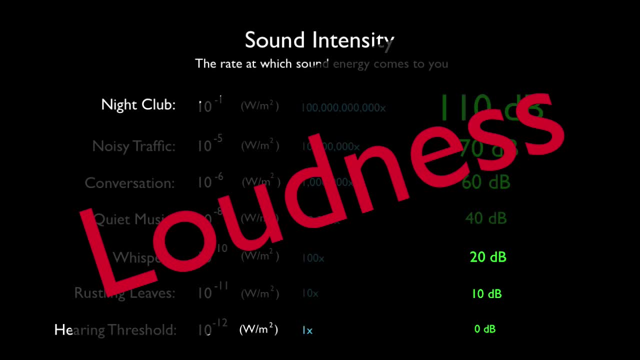 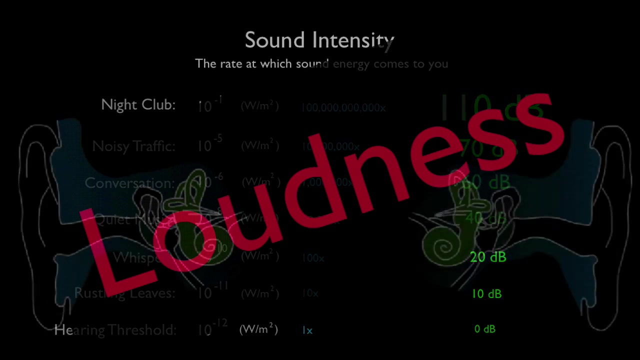 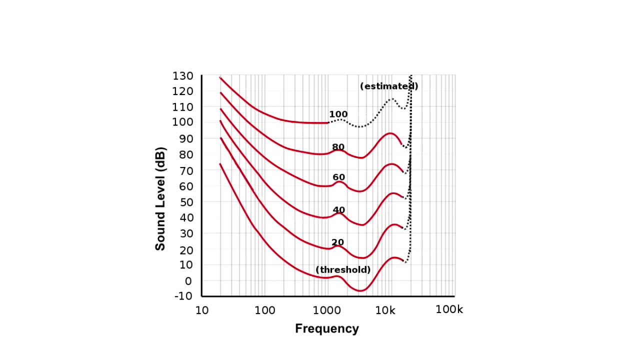 there's still a lot of biology at work in our perception of that sound. Generally speaking, the more dB, the louder it sounds, But not always. You see, the human ear is not equally sensitive to all sound frequencies. Take a look at this chart plotting sound intensity to frequency. The curves are called. 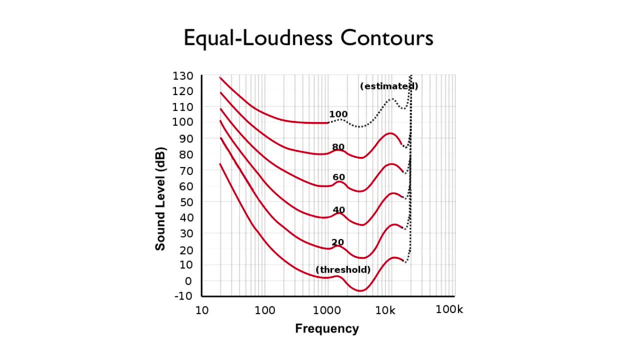 equal loudness contours. Say, you're listening to 1,000 Hz at 20 dB, You'll hear it to be so loud. Then someone starts playing a 100 Hz sound. Now how many dB are needed so that you hear the 100 Hz just as loud? 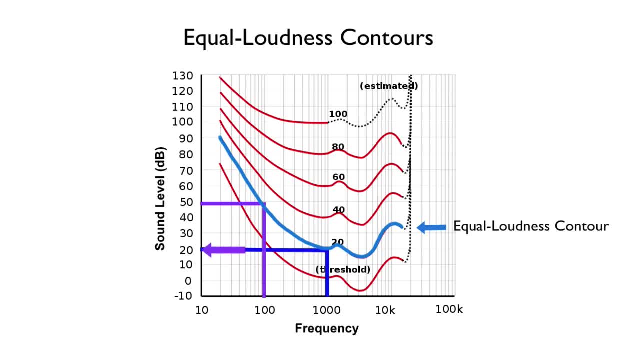 You might think also 20 dB Here. listen to this. I've got 1,000 and 100 Hz playing at the same intensity. We're much better at detecting 1,000 Hz than we are at detecting 100 Hz. That's why you're likely hearing the 1,000 Hz as being louder.